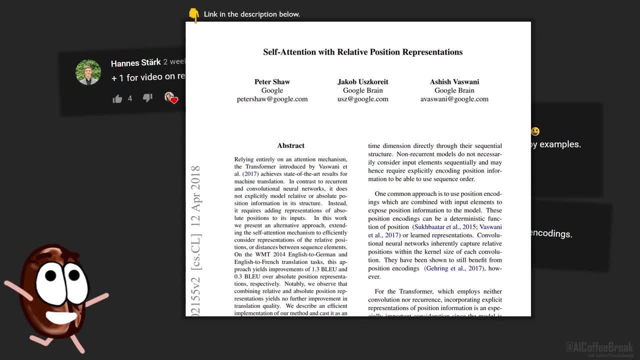 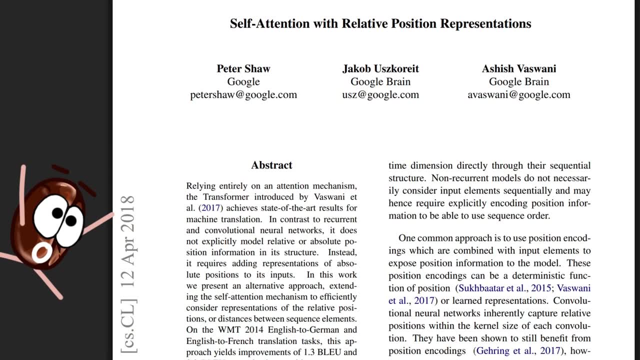 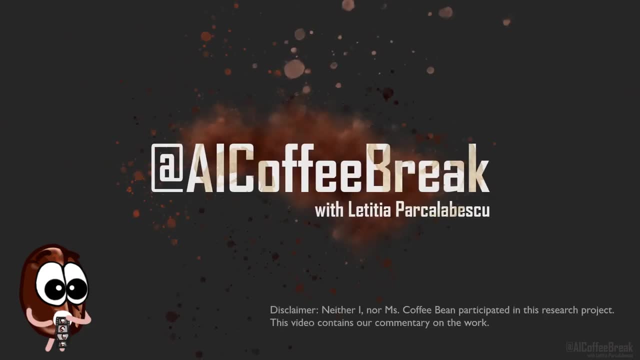 Hello, there It's finally here, the long-promised video explaining relative positional embeddings as they were introduced in prehistoric times by our ancestors in machine learning. So if you're not yet sick of positional embeddings in transformers and want more of them, you are spending your coffee break with the right video, Because, well, we did a video about. 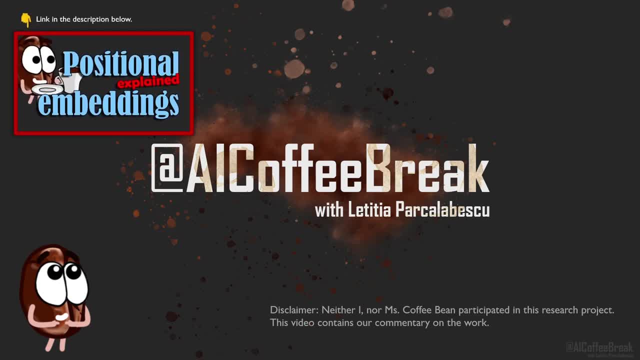 positional embeddings as we introduced by the. Attention is all you need paper. then we had a video about concatenating vs adding positional encodings and there we also discussed learned positional embeddings. This coffee bean is now literally 50% caffeine and 50%. 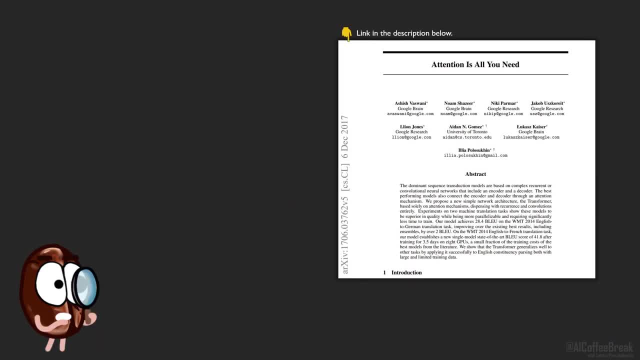 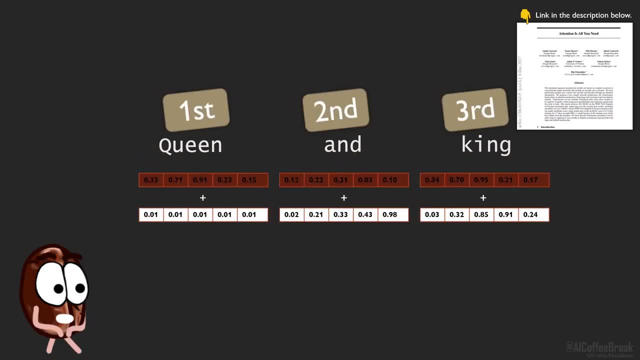 positional information. Let's begin. The Attention is all you need. paper introduces positional embeddings that encode the absolute position. They encode the exact order of topography, the inconsistency of cylinder DIRECTORY Lorentz, the consistency of C色 Day last talk形ound lobby and a lower dead space. helpще, We forgot the function to name them. 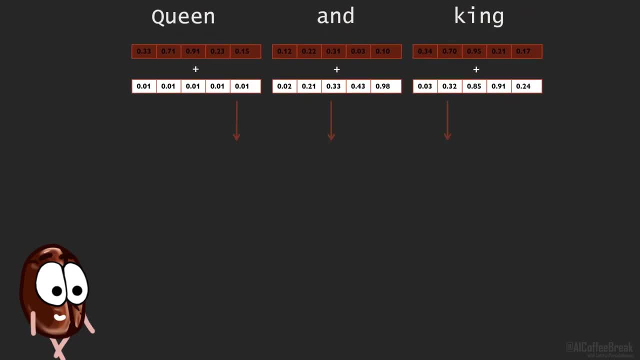 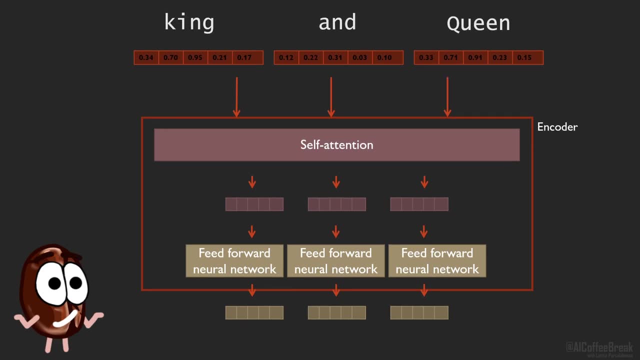 There are additional questions, leave the comments. I recommend watching. couldn't do that. You can also token such that the transformer is informed about the sequential nature of data. Otherwise, the transformer that is processing everything in parallel would be invariant to order, meaning that without positional encodings its output would not change after. 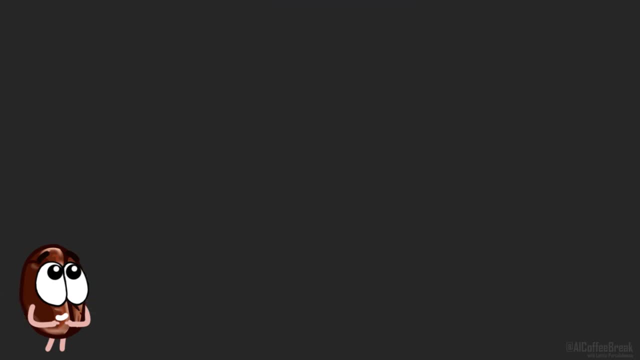 complete sequence reordering. But what if we are dealing with other kinds of data where it is not about absolute position but about relative positions? Think about a graph, for example. It would be quite arbitrary to say that a certain node is the first one. what would 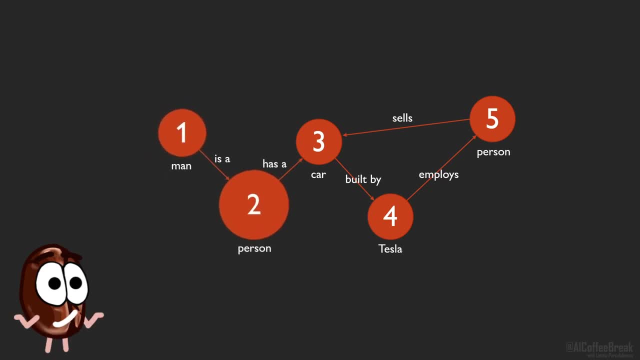 make this node the first node and this the second. That would be unmotivated for many problems and in some cases even misleading. Then let's forget about absolute order and move to relative positional encodings that are about the distances between elements in either a graph or a sequence. 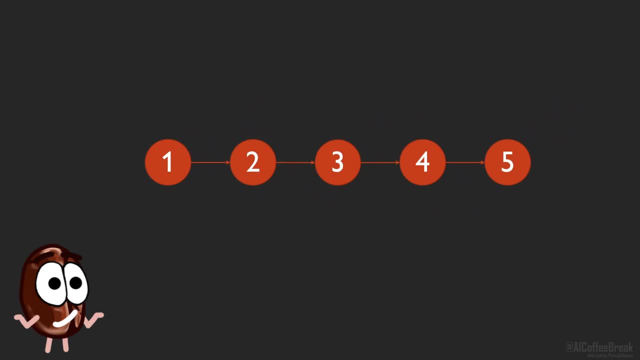 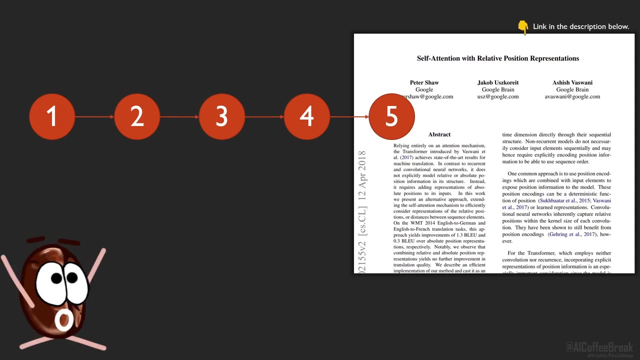 Which is in fact the same thing. A subset of the authors of the Attention is All You Need paper also have a follow-up paper doing exactly this. They introduce relative positional encodings where not the order but the relation, or, better said, the relative position, the distance between tokens is important. 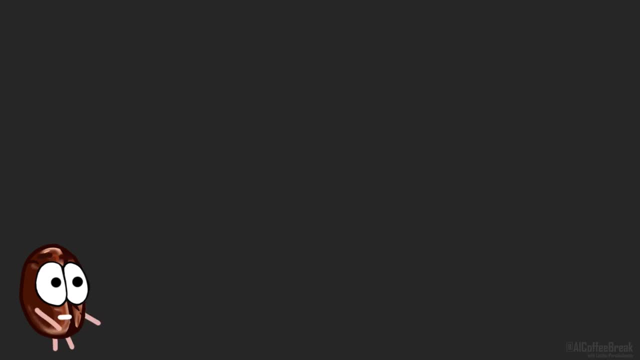 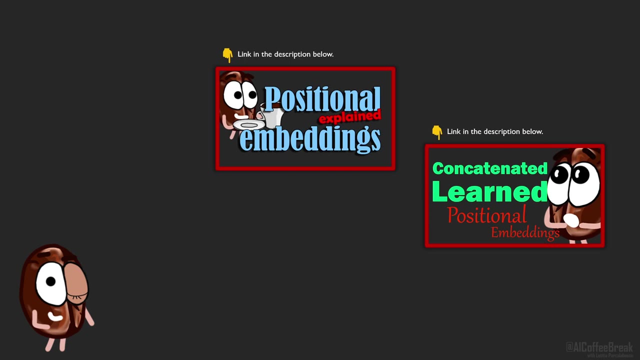 So how does this work? If you do not know anything about positional embeddings, first go and watch our two videos about them and then come back. Don't worry, they're short. The idea of relative embeddings is moving away from the classical positional embedding. 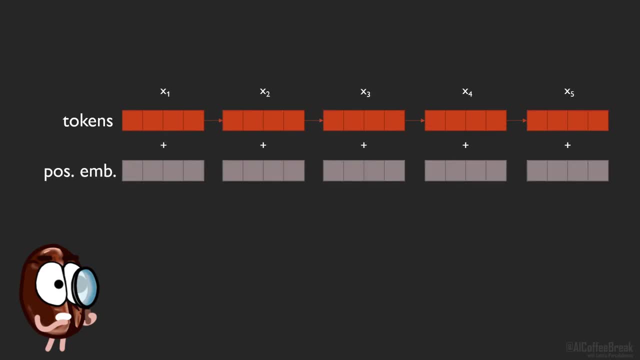 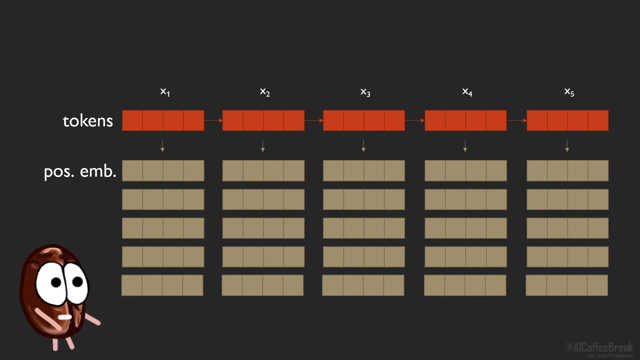 where each token has its own positional embedding. With relative representations, each word or token does not have only one positional embedding, but as many positional embeddings as there are tokens in the sequence in order to describe the relationship between them. This is because relative positional representations do not encode a single positional embedding. 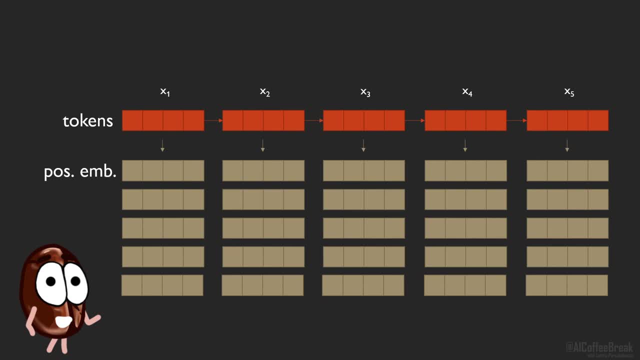 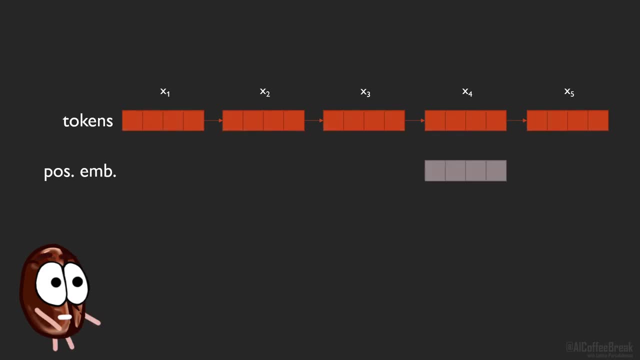 or an absolute order anymore, but a positional relationship in which each token stands to the other tokens. So let's take an example sequence of five tokens In classical positional embeddings. each token- let's say X4 here- has one encoding informing: 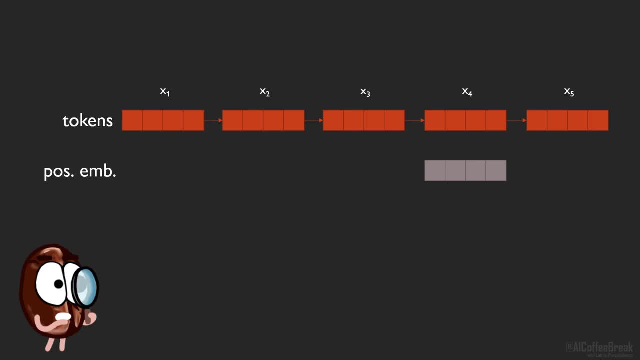 the transformer about the position of X4.. Now, to best visualize relative representations, let's copy the sequence again like this: Let's copy the sequence again like this: In the relative variant, each token has five positional embeddings: One embedding for describing its relative position to itself, then four others for the 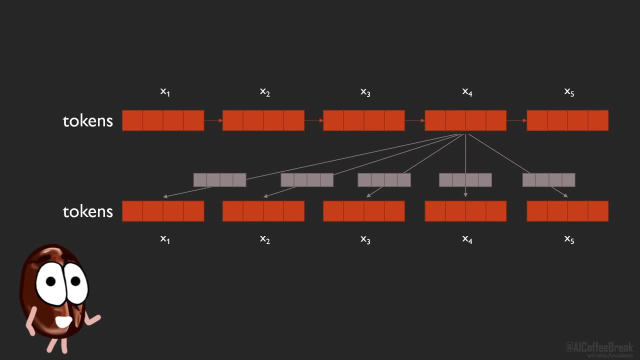 rest of the sequence And to keep the same notation as the original paper, the positional embedding describing the relationship of one token with itself is a vector W0, as 0 is the distance between the token and itself. Then W1 and W2 as we move to the right. 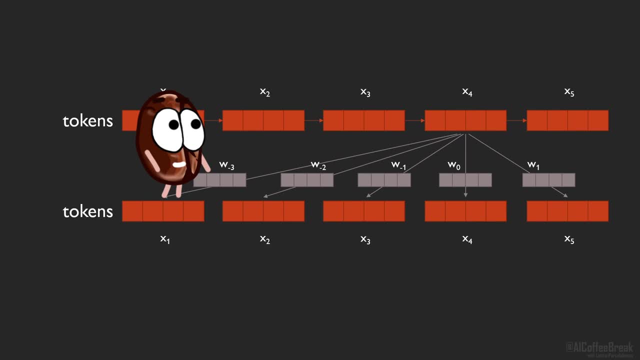 And W-1 as we move to the left, Then W-1, W-2, and so on as we move to the left, And the vector WI takes the same value, independently of what tokens we are currently looking at, Because W0,, wherever we are, says that we are at zero, hops away in the graph. 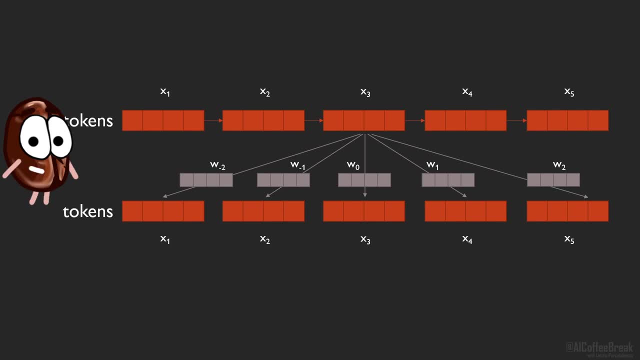 W1 says that we are one hop away to the left in a sequence Or in a directed graph. in general, we go one hop following outgoing edges. So you see, This approach is not made only for sequences, but for graphs too. Okay great. 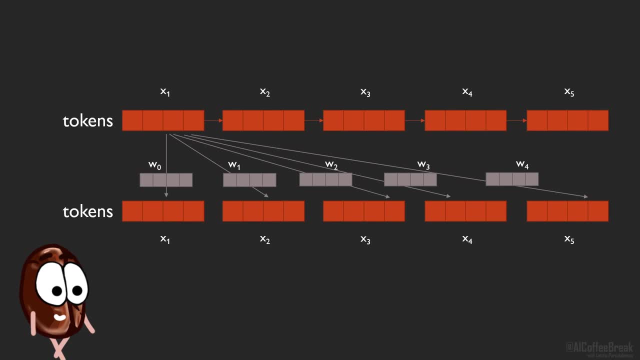 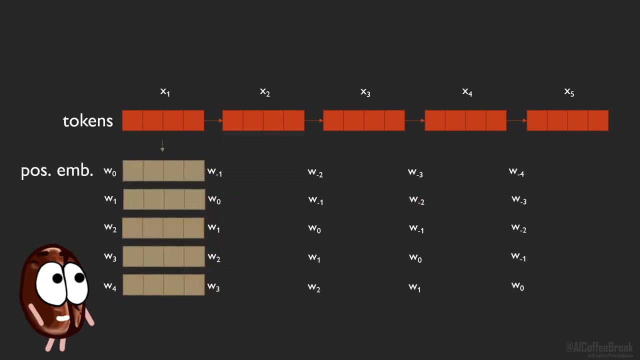 For a sequence of length 5, positional embeddings should range from W-4 to W4.. So we have in total 9 positional embeddings to either handcraft or learn. for this sequence, These W vectors can be written one under the other in a table like this. 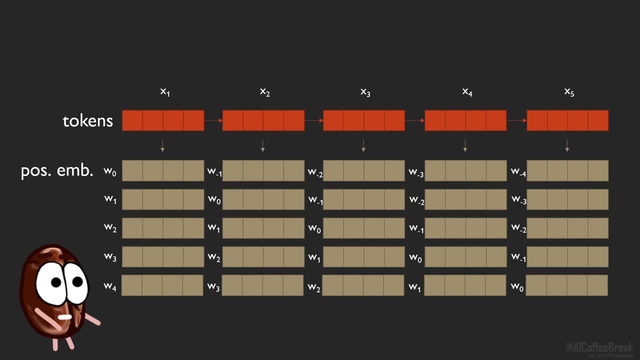 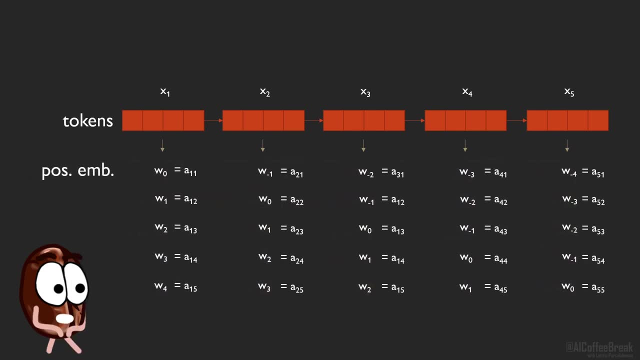 Notice that these vectors come from the relationship or distance between one token. So we have W1,, W2, and W3. So we can use a pairwise notation for this. The authors also experiment with clipping at K, meaning that after a certain distance. 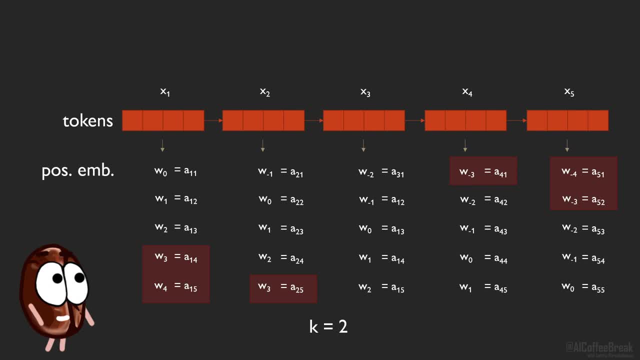 positional embeddings get the same value. So for K equals 2, W3 and W4 all take the value of W2.. Okay, but now for each token we are stuck with as many positional embeddings as the sequence has tokens. What to do with all of these? Add them all up. That wouldn't be a great idea. Addition is complicating things even with sinusoidal embeddings where we have just one positional encoding for each token, because we could mix up the semantic and positional information. With 5 positional embeddings per token, the mixing up problem would be only 5 times larger. 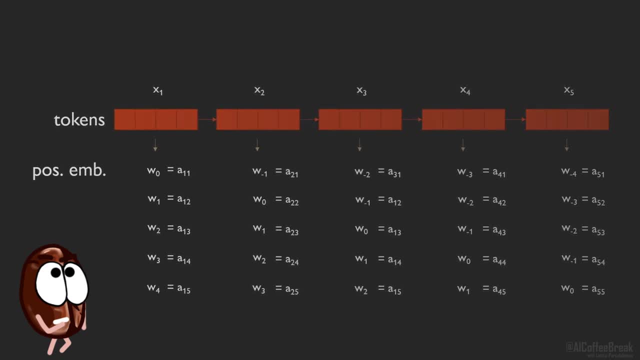 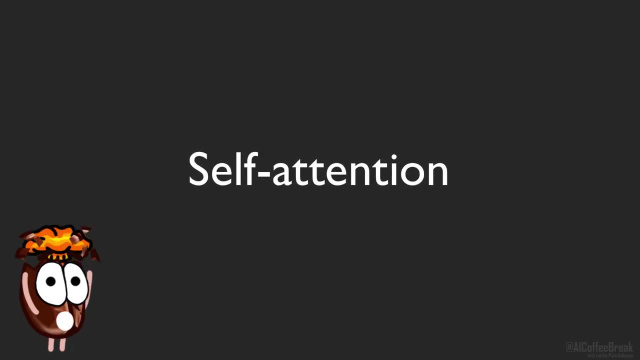 If only we had a mechanism that, given a token, computes new representations for that token in relationship to all other tokens. Heh well, we do have this. It's the self-attention mechanism. A clever idea would be to modify the self-attention. 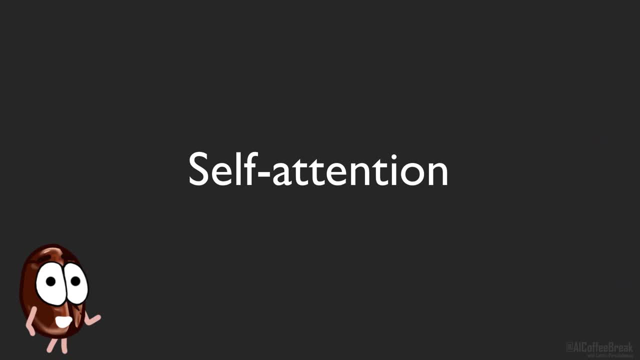 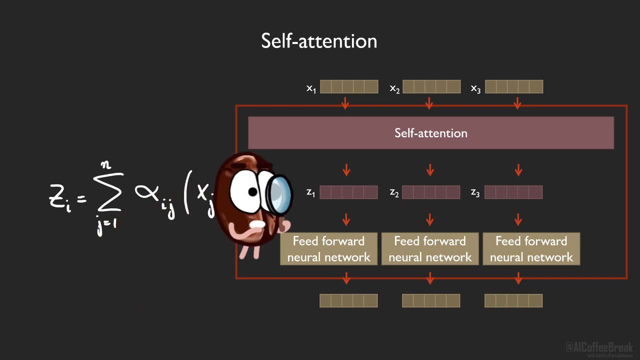 formulas to capture the relative positional representations too. We remember that through self attention each token gets a new representation, Z, which is passed further in the transformer module. Each token vector is first transformed by a linear transformation, then the new representation for each token will be changed. For example, each token vector is the first transformed by a linear transformation, Then the new representation for each token is implemented by a linear transformation, Then the new representation for each token is adopted. 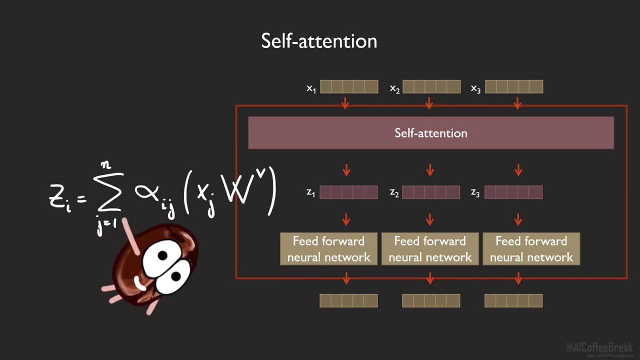 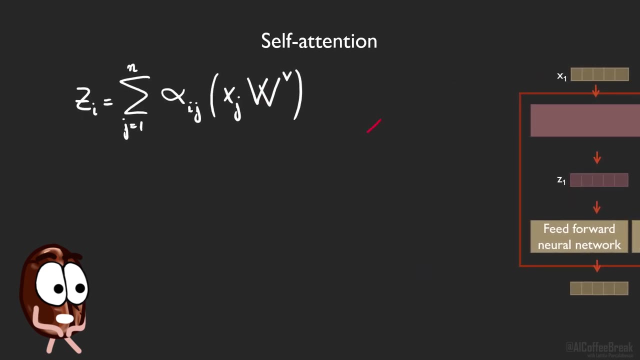 token is a weighted sum over all tokens where the weights are sort of an importance score. So fellow tokens that matter more are weighted more. So here, where the new representations are computed, we can add the positional information. Now the token representation after the linear transformation is: 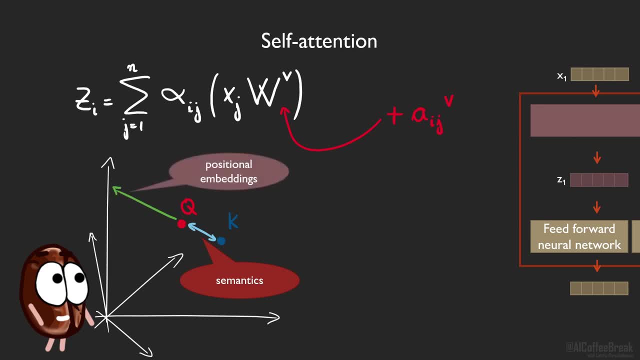 further shifted in the high dimensional space. This means that each token XJ gets pushed into a subspace, saying that: look, I carry this semantic information, but I'm also your second neighbor to your right because my position in some dimension is similar to all other second neighbors. Okay, Great. Now the new representation Z. 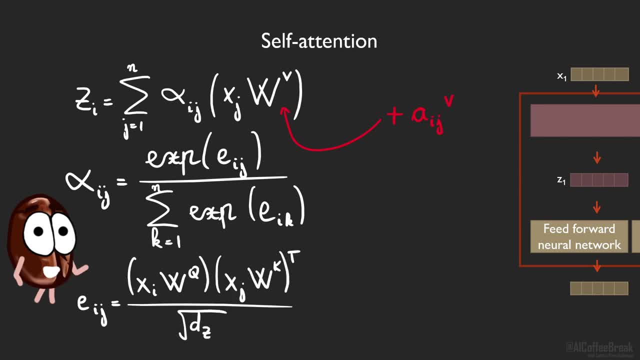 is informed about the relative position, but the self-attention weight coefficients are not. Therefore, the weight coefficients also receive their own positional push, such that they are not related to each other. The important scores make positional informed decisions too. So what do we have? 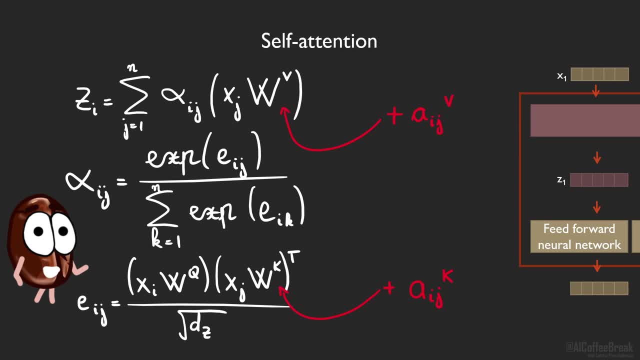 in the end. Now every token has as many relative embeddings as there are tokens in the sequence in two variants: One relative embedding for the values and one for the keys to inform the attention. weights And the exact values of the vectors are learned, which kind of makes sense to let the model figure out for. 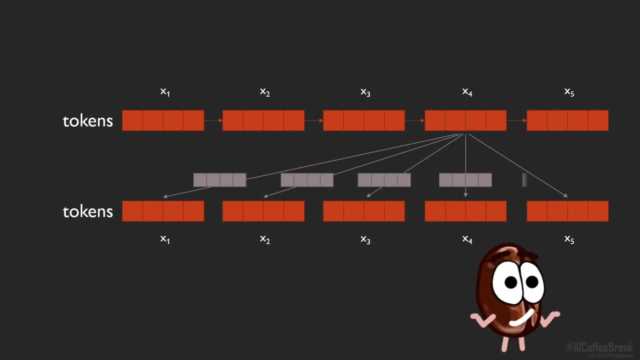 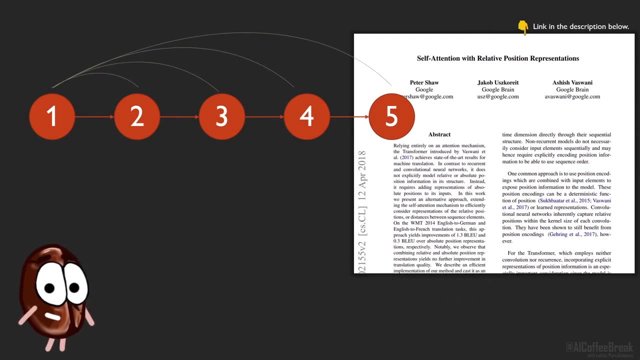 itself what the best balance is. It would be interesting to see how this works out. It would be quite difficult to handcraft all of these. And what did this whole thing help with? Well, this paper has only experimented with text, which is a sequence, obviously, and they gain some performance in machine translation. 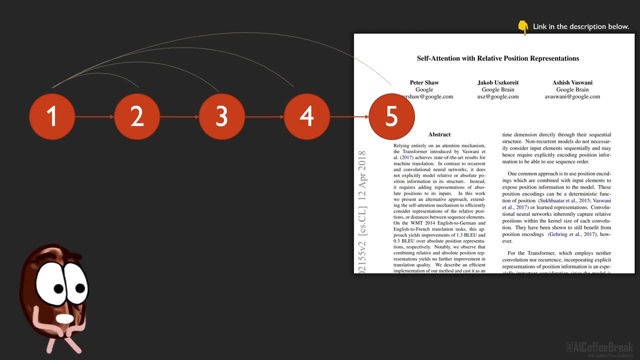 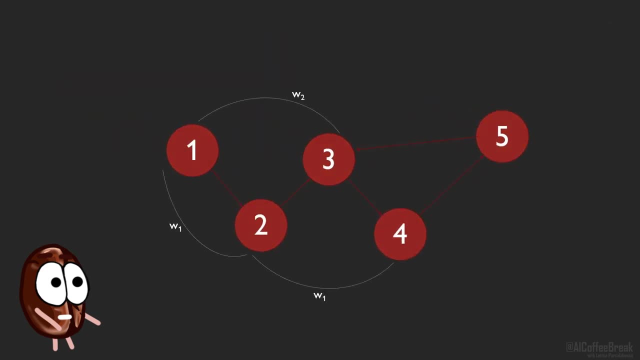 But word chains are only a flat graph And beyond this, the method can be applied to graph representations in general or anywhere where you have pairwise relationships between your elements, Because, remember, these relative representations depend only on how far tokens are from one another, independently of whether 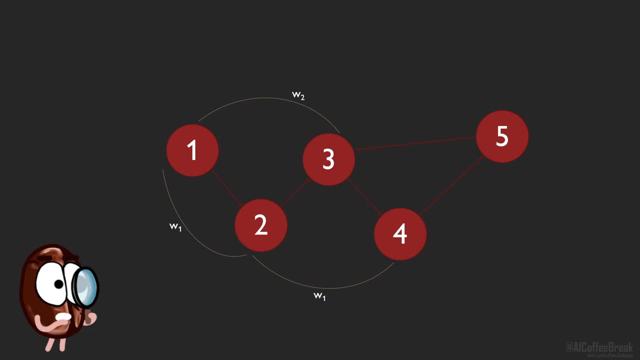 we are in a sequence or in a more complex graph. But, Ms Coffee Bean, why didn't this paper try this out immediately? Well, it's called marking your territory, But there are other papers that implemented this successfully for graphs too. Anyway, another upside of relative positional 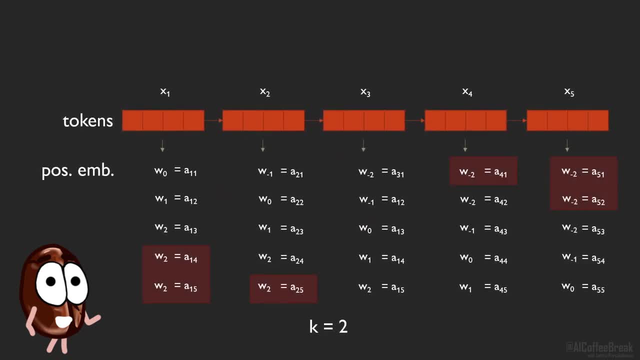 representations is that, especially with clipping at K, this learned positional information generalizes to any sequence length, which is also a feature of the handcrafted sinusoidal embeddings but not necessarily of any learned positional embedding. Clipping at K seems a little odd because with small k it takes away the information. 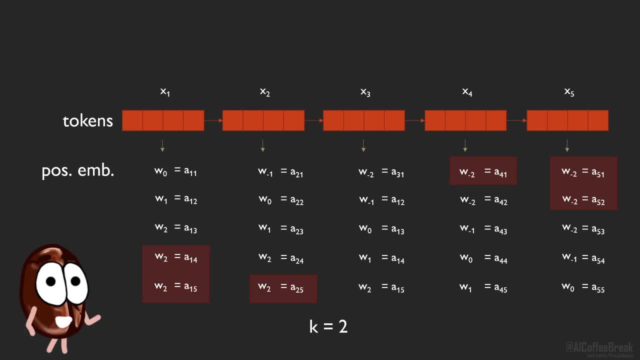 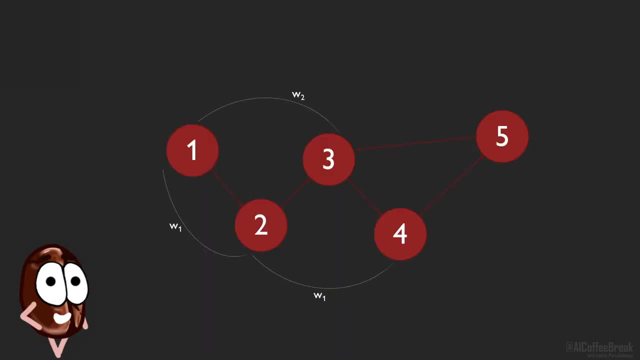 of long-term dependencies. Now we can only store that something is close by or far away, but we don't know how far away that is. But this is similar with graph neural networks, where the best results are delivered with a small number of iterations.